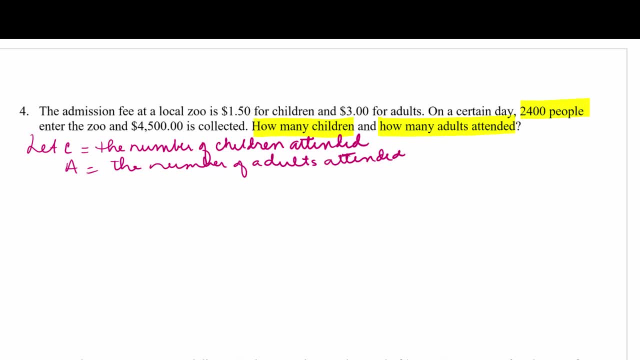 And there were 2,400 people total. So that tells us that the number of adults that attended added to the number of children that attended that day has to add up to 2,400.. So that's our total, isn't it? 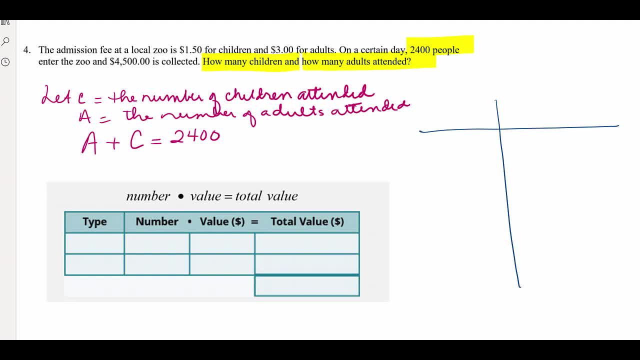 Now, to help us set up the second equation, we've gone ahead and brought in this table. You may recall that we used a similar table back in Chapter 2.. The type of tickets that we're selling here are that we have adult and we're calling that number of. we're representing the number of adult tickets sold that day by A right. 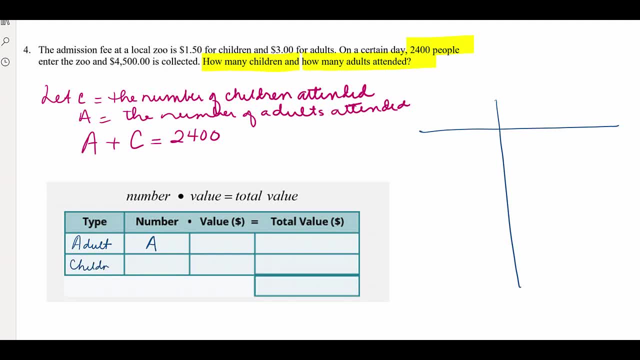 Because those are the number of adults who attended And we have children. These are the people going to the zoo And we're representing the number of children. with C, The value of each adult ticket is $3.. And the value of each child ticket is $1.50. 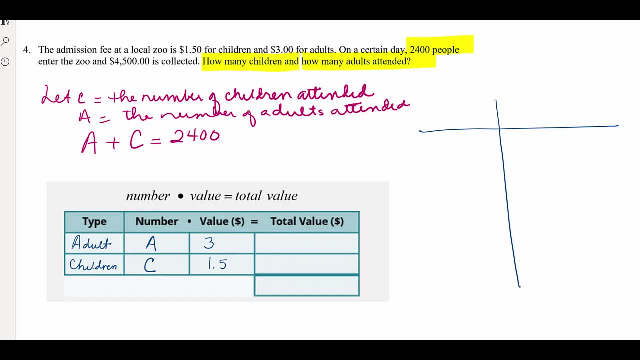 So I'm going to put 1.5.. And then the total value then that we collected or that the zoo collected that day in adult tickets sold is found by multiplying the number times the value, so 3A. And then the total value that was collected in child tickets is also found by multiplying 1.5 times C. 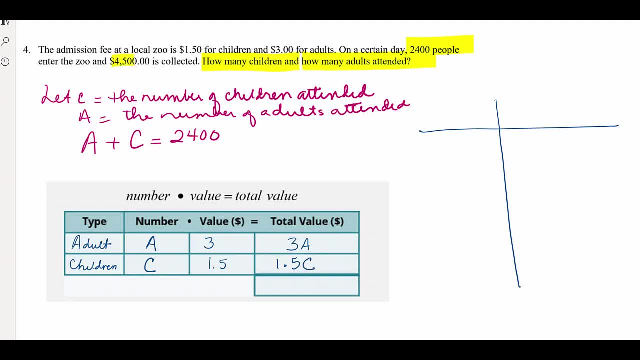 And we know we were given that That total value collected was $4,500.. So $4,500 goes here. And then, in this last column we've got our second equation, which I'm going to put over here in my T-table, because I've already decided that I'm going to use substitution method. 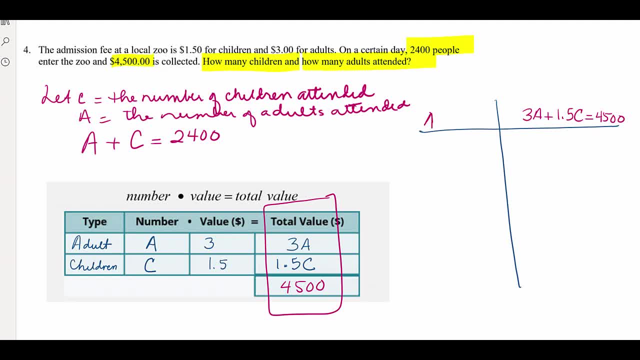 And why did I decide that? Because I like this first equation. It looks pretty easy for me to solve that for one of the variables. So now I get to choose. which variable shall I solve for? And I think I'm going to solve for A. 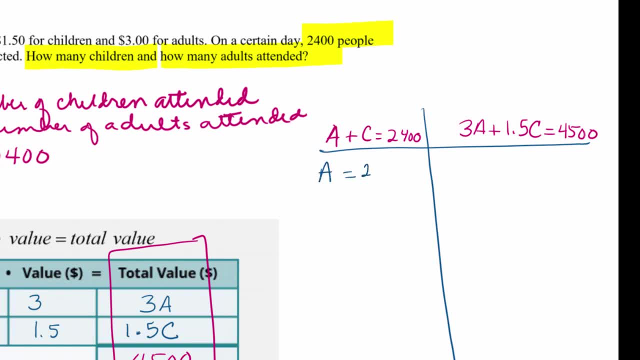 So we get A equals 2,400 minus C, And I'm going to take that expression here on the right-hand side And, as you know, I'm going to bring this over here to my second equation. I'm going to substitute it in where that A is.